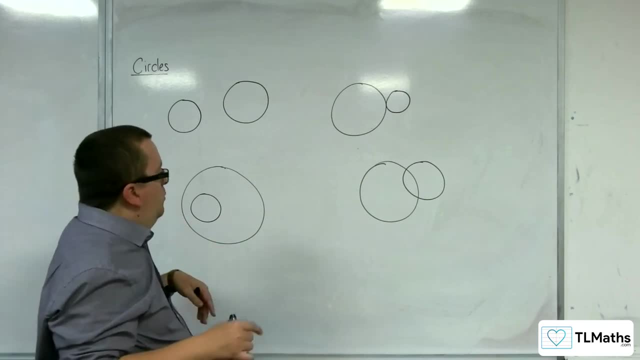 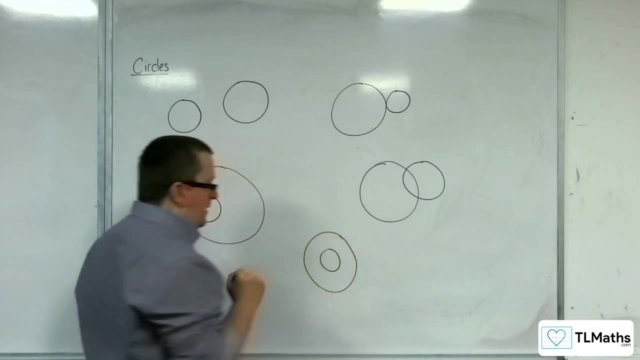 We can do that. How can we tell which is which? Well, I've actually missed one off, haven't I? I mean you could have? I did mention concentric circles, okay, Which is kind of like this situation, But we'll explain the difference. 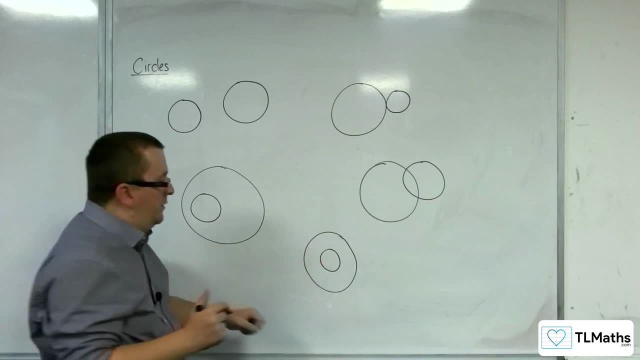 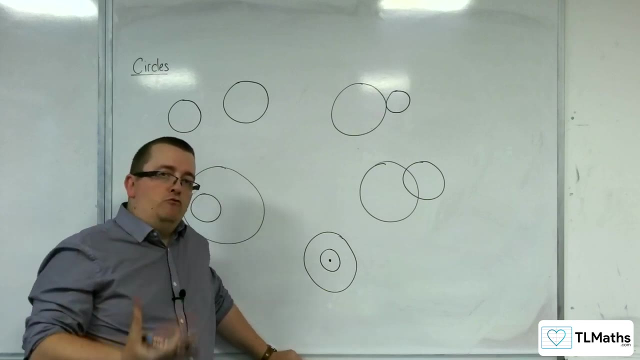 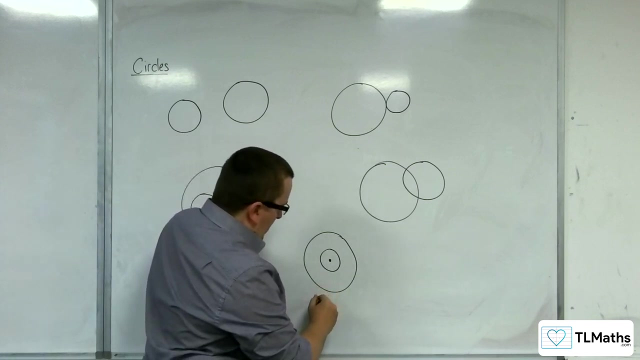 So if we go, let's have a look at this one first, then this concentric circles. I mean, the idea here is that they both have a common centre, okay, But they have different radii. So if we use the, let's say, let's call C1, right? 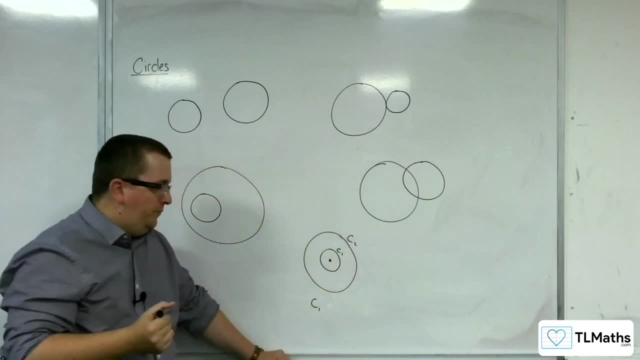 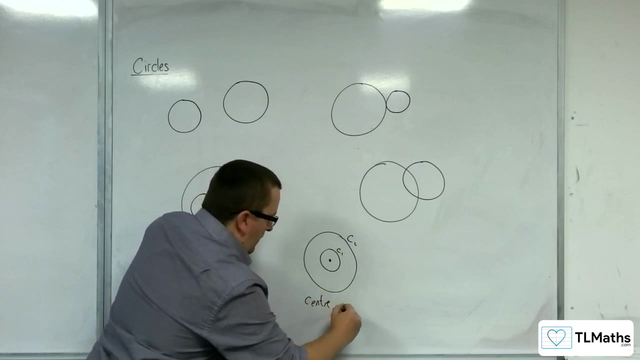 This could be C1, and this can be C2,, okay, So. Okay, So centre 1 is equal to centre 2.. So the coordinates are the same, but the radii are different. then we would have that situation. 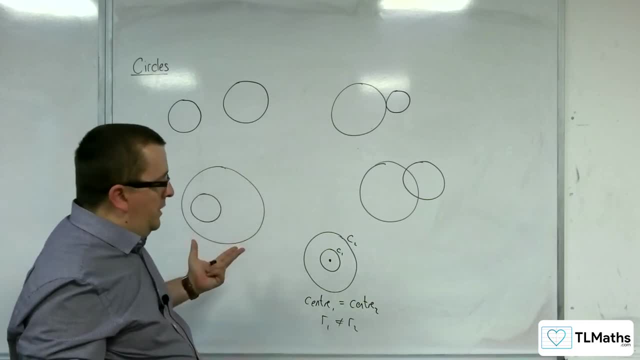 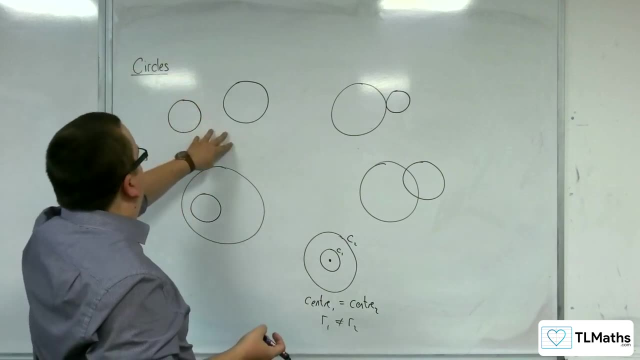 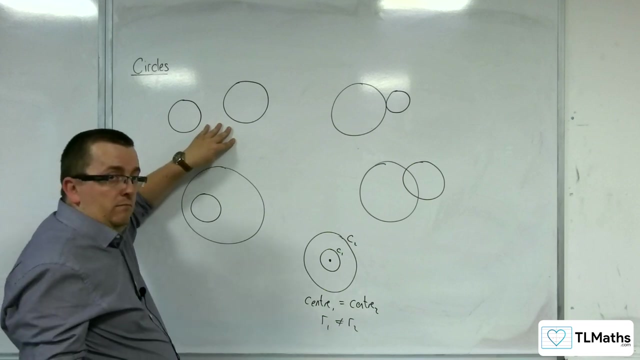 So they both have the same centre, but the radius is different. okay, That defines concentric circles, Okay. so let's say we've got this then, okay, We've got two different centres, clearly. Okay, But the radii could be the same, they could be different. 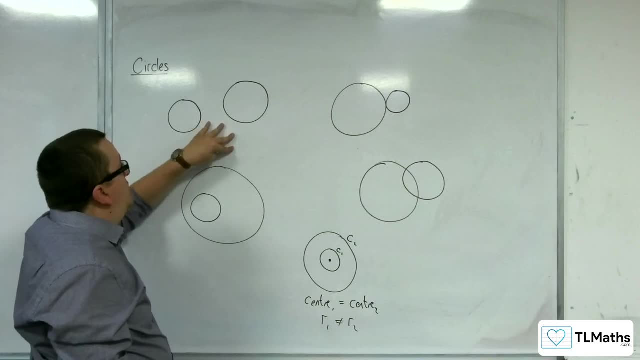 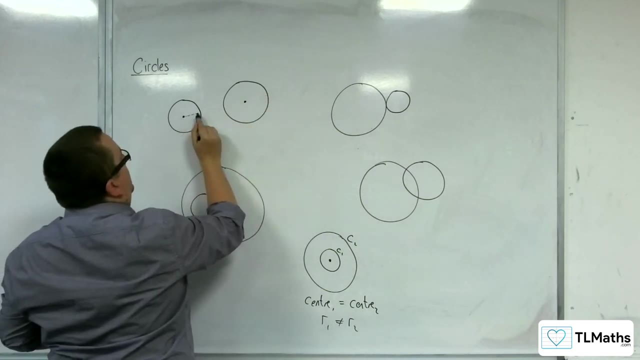 So how would you show this to be the case? What would be the result? Well, if you worked out the distance between the two, we could call that D. okay, If the distance between the two centres is greater than one of the circles' radii, then 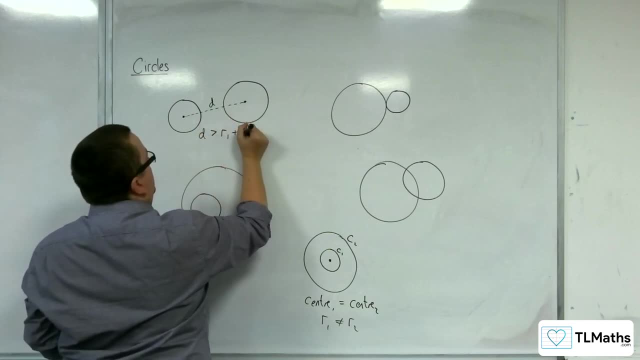 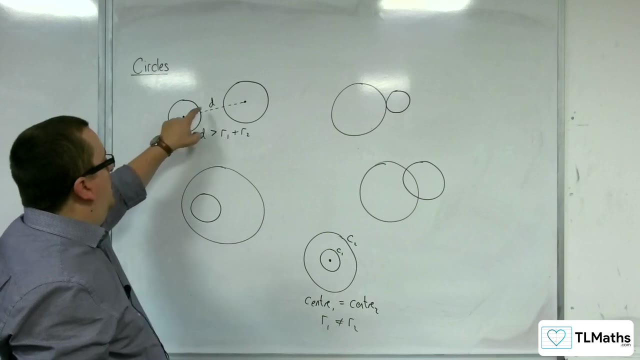 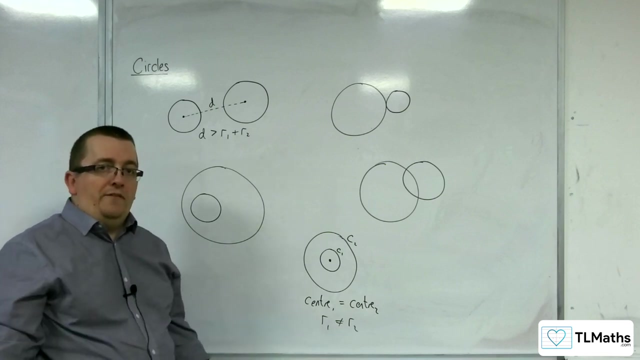 plus the other circle's radii, then we must have that situation, okay? So if this has got a radius of 2, this has got a radius of 3, and the distance between them is 7, okay, Well, 7 is greater than 2 plus 3, so they can't intersect one another, okay. 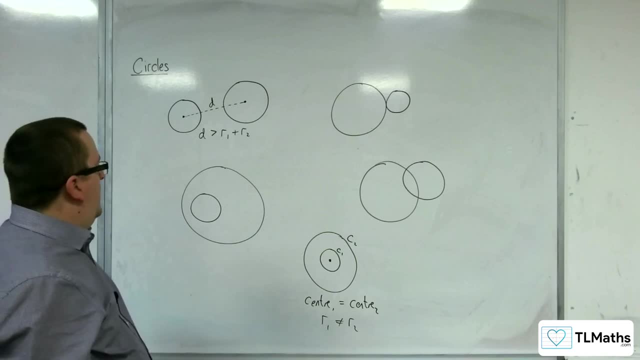 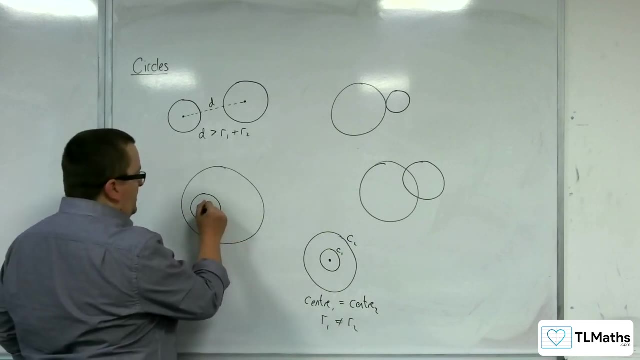 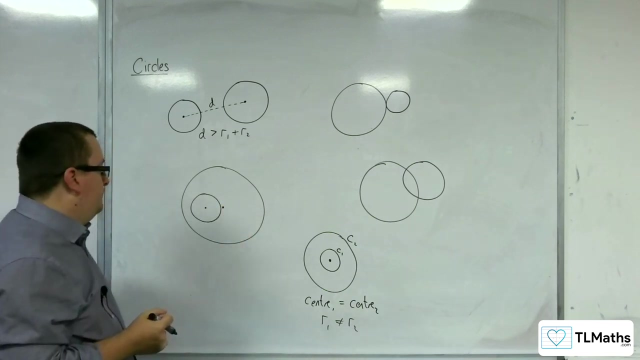 Right, How about this one? Let's have a look at this one now. Let's have a look at this one next. So this one: the centres are different. okay, So that's part, maybe the centre here. okay, So the centres are different. 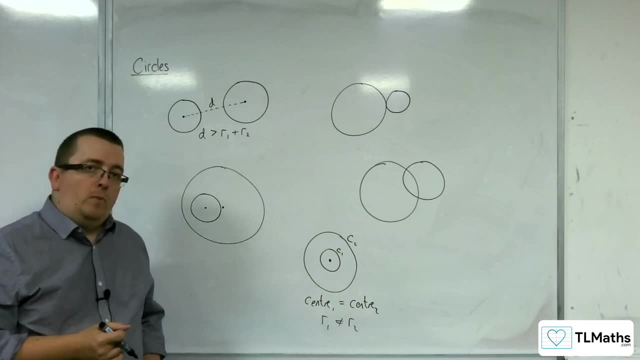 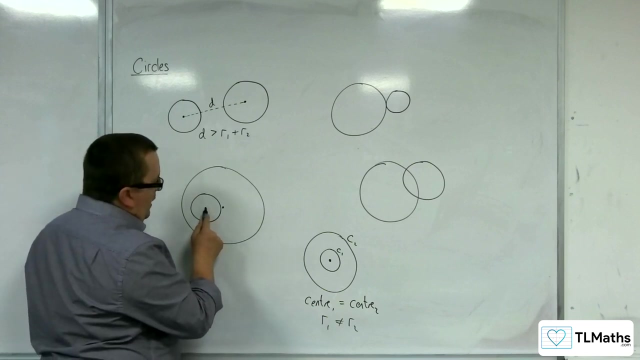 How would you determine that we don't have intersecting circles or one is completely within the other? Well, if you think about it this way, Okay, We'll probably be looking at how far the two circle centres are away from one another. 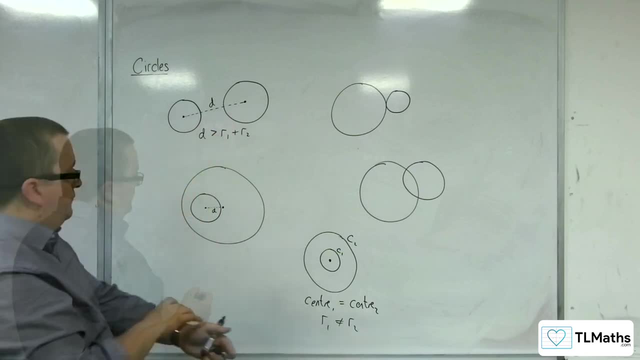 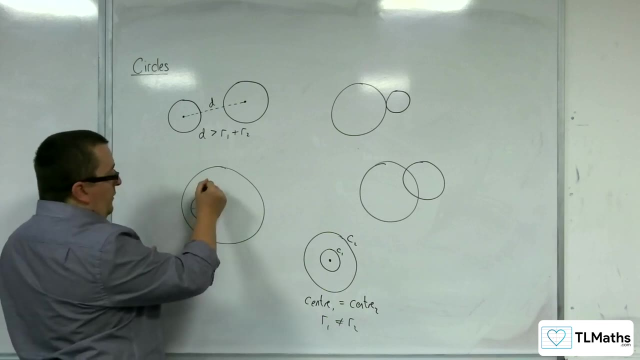 Let's call that D, like we did up there. Now we could also put on our diagram that this distance here is R1.. So we'll call this circle 1 and this circle 2.. This one was circle 1,, for example, and that was circle 2.. 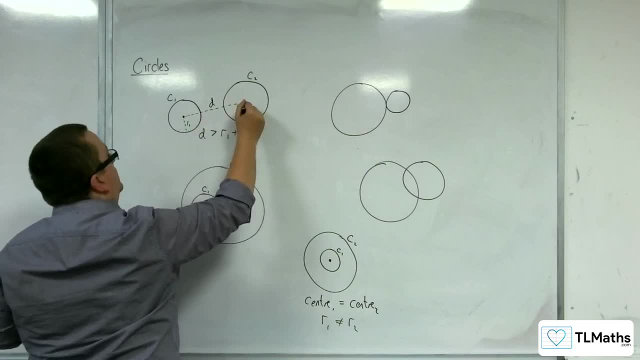 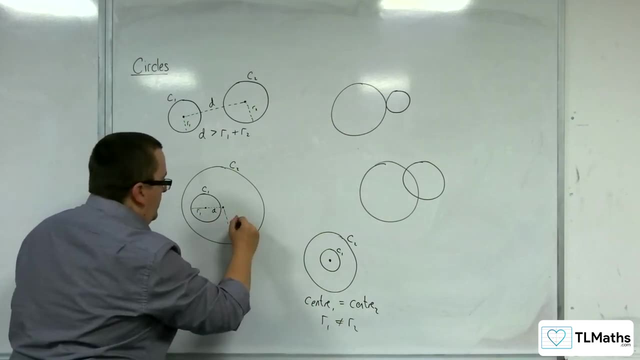 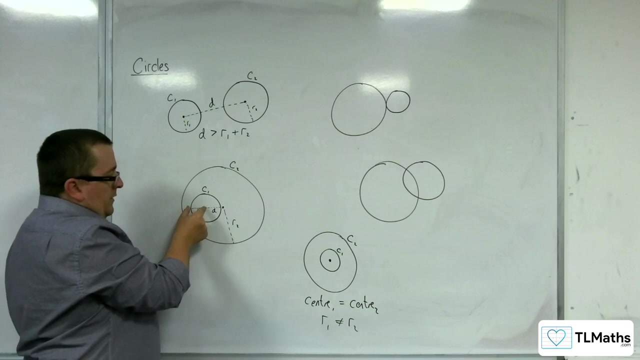 So R1, R2, just to kind of keep some order about things- And this is radius 2.. Now if that distance plus the distance of R1,, if that's less than the distance of R2, then you know that circle has to be within. 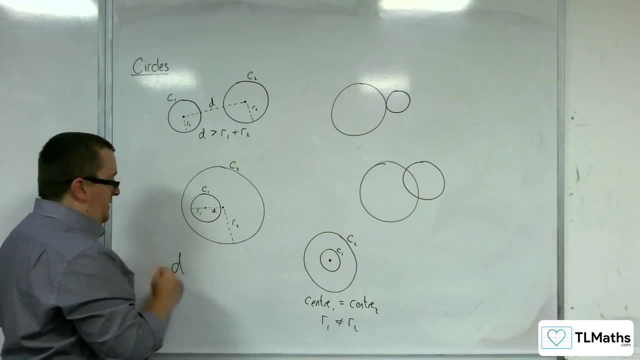 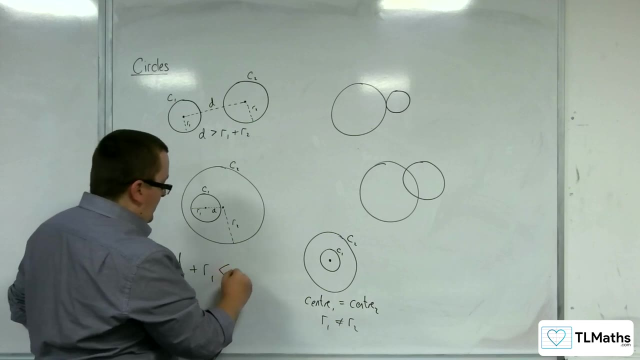 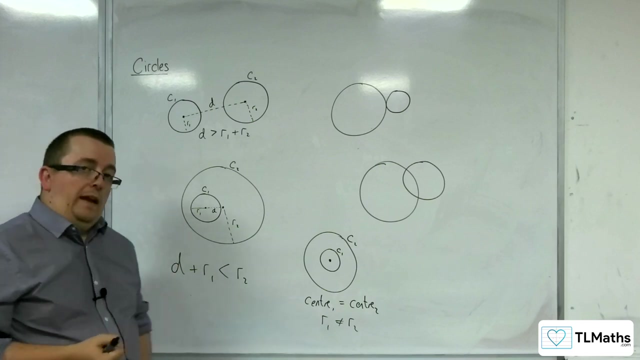 So if And The distance between the two centres plus the radius of the smaller circle inside is less than the radius of the circle of the larger circle, then one circle would fit inside the other. OK, So this would also be the case. 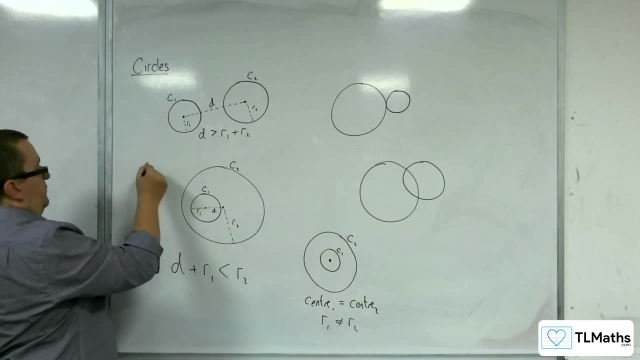 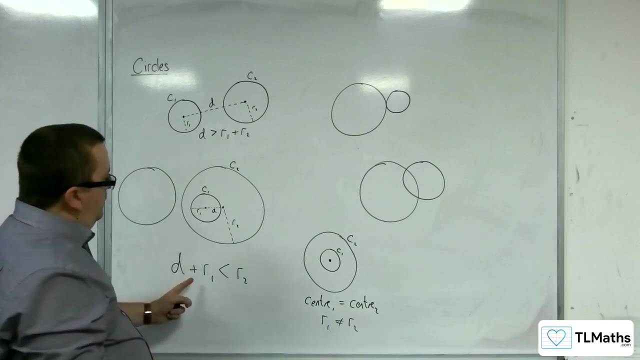 I mean you could draw it in an alternative way, so that I mean it's effectively. I mean, if you thought about it like this situation, the distance here between the two centres is zero And you're just saying that R1 is less than R2, which it's got to be for the concentric circle. 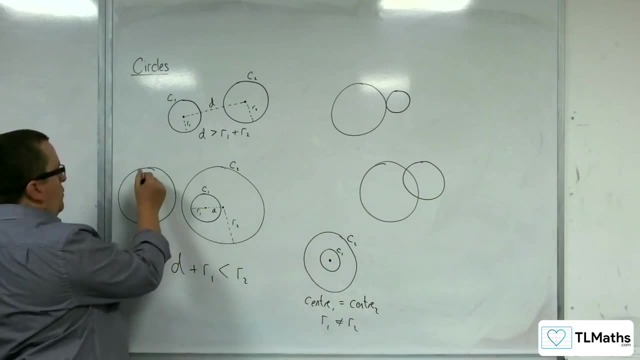 OK, So it does fit this as well. I mean, if you drew maybe quite a large circle, OK, Here's the centre of the exterior circle C2. And here is the centre of the smaller circle, C1. Then if that distance 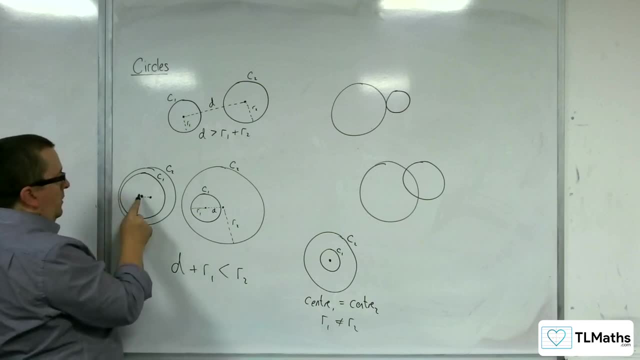 OK, Plus that distance is less than R2.. OK Then, as you can see, that distance Plus that distance, If it is less than R2, then you're within OK. So it might be easier to kind of see it from that diagram rather than that one. 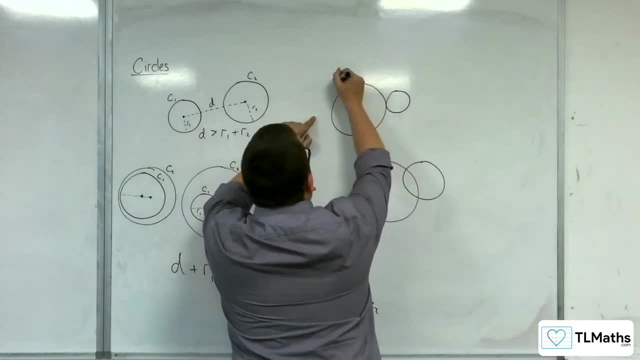 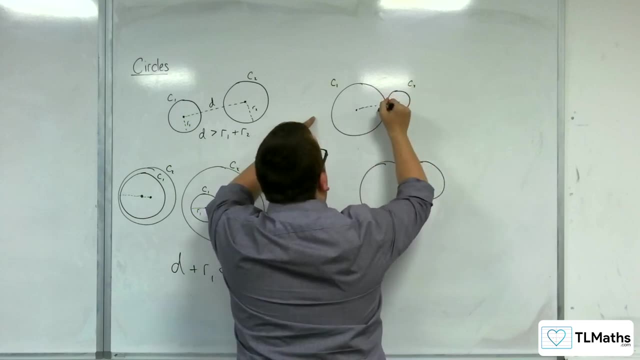 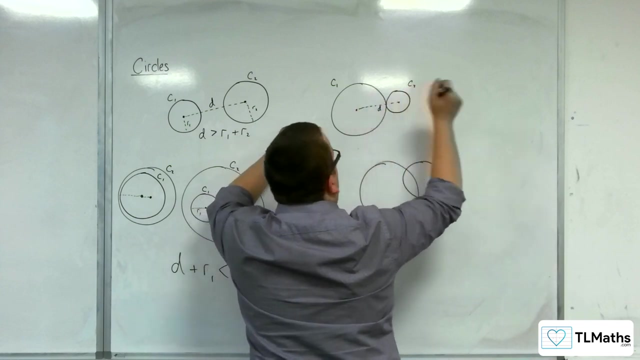 Let's go up here then. OK, So here is: Let's call this C1.. And this one is C2.. OK, Here is the distance between, And you can see that the distance here is actually the same as R1 plus R2.. 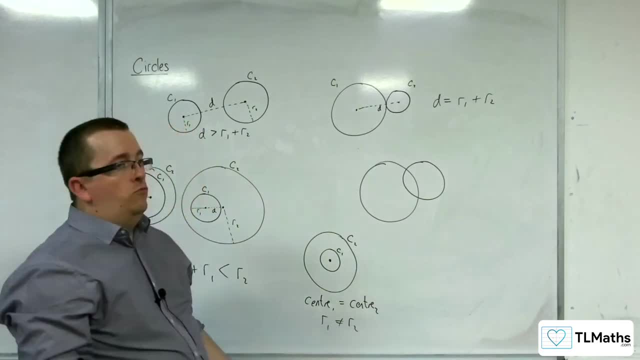 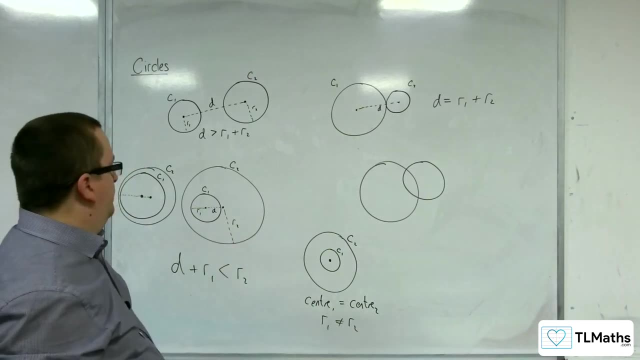 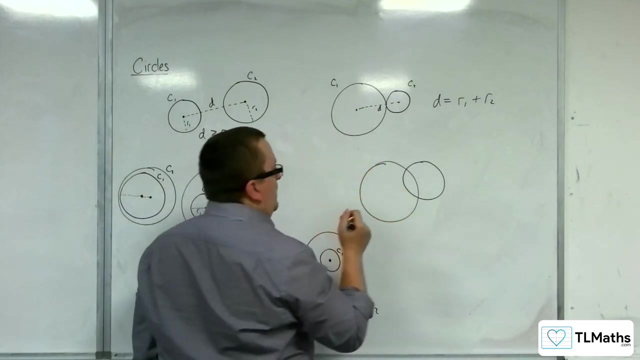 So if the distance is equal to the two radii added together, then they must be tangent to one another. OK, They must just touch each other. at that one point, This situation where we've got two intersection points, we've got this overlap. 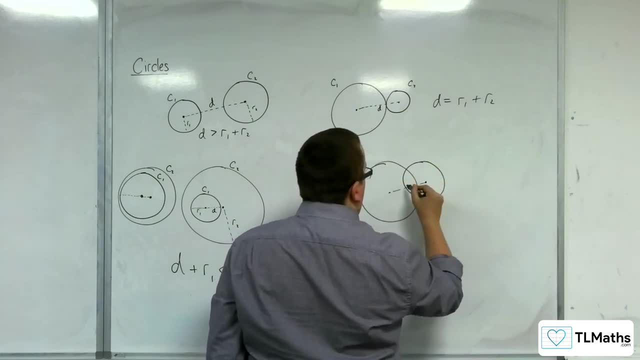 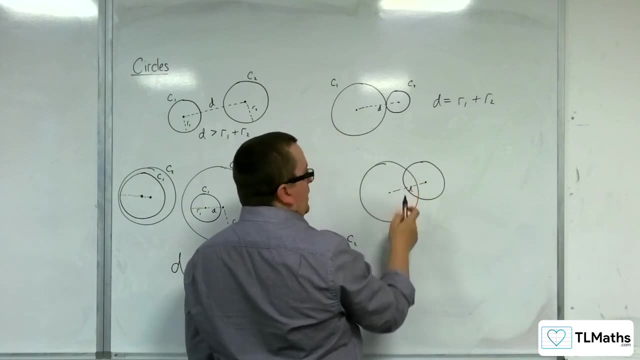 OK, Here's my centre, Here's my centre. Here is D. OK, You can see here that D must then be less Than the sum of the R1 and R2.. OK, Because that's R If that's C1 and that's C2.. 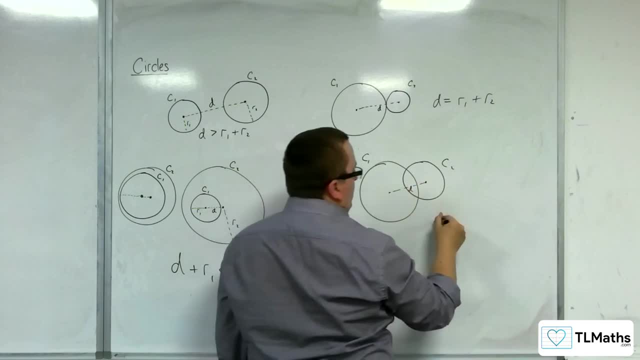 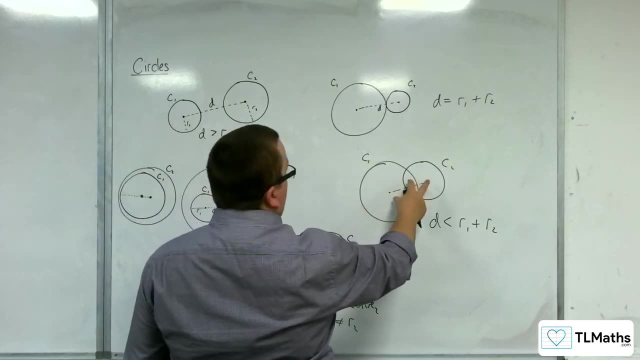 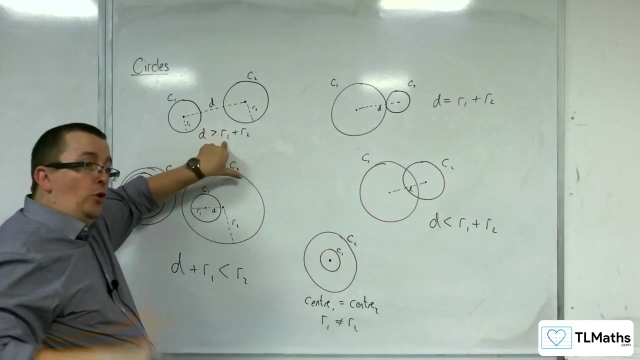 This is R1.. This is R2.. So D is clearly less than the sum. So if it's less than the sum, we have this intersection. If it's equal to, we have the tangent. If it's greater than, we have this kind of two disjoint circles. 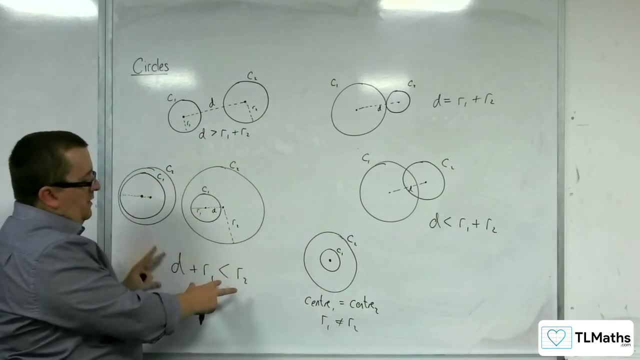 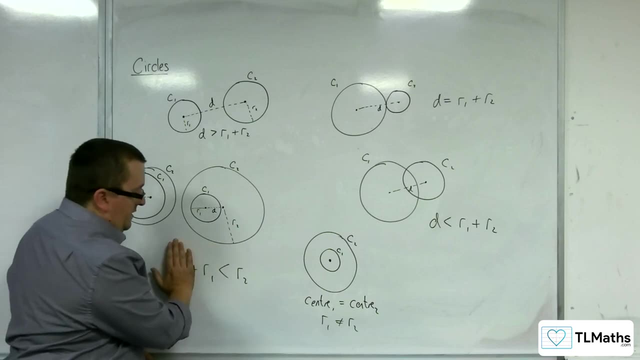 OK. And if? If one is inside the other? we've got this situation here, Which also works with the concentric circles, If you just imagine. well, the distance is zero. So these are the situations that you can deal with. 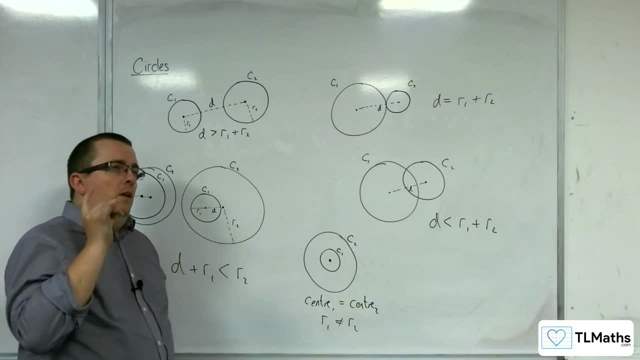 OK, And it's just thinking about if I was given two equations of circles, if I could work out their centres and I could work out their radii, then, using that That information I should be able to work out and visualise. 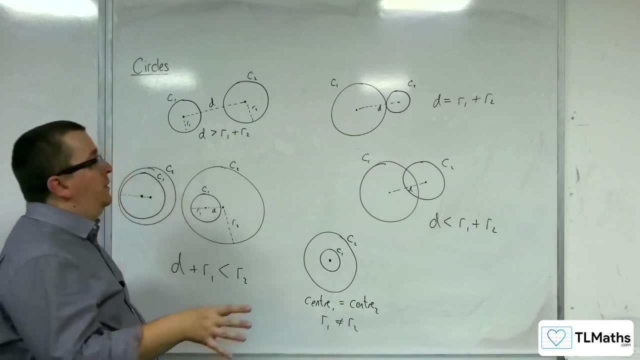 and I'd always suggest a diagram whether the two circles intersect or don't.